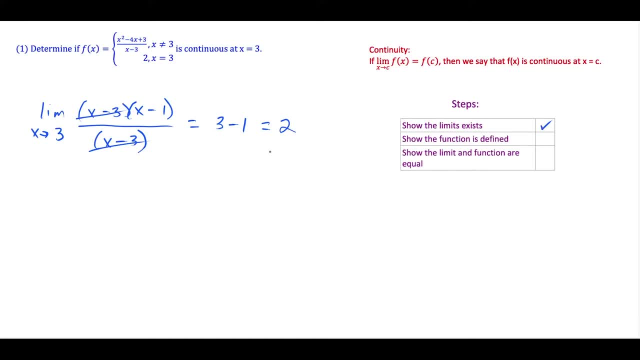 which is equal to 2.. So the limit does exist. So this is a good start for us, showing this function is continuous at x equals 3.. But now we want to show the function is defined at x equals 3.. And if we investigate f of 3, this is just the point 3 comma 2.. So the function value at 3 is equal to. 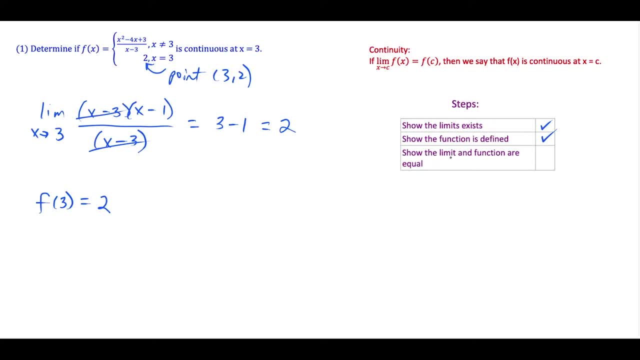 2.. So this is also checking out here And now. the last thing that we have to be able to show is that the limit and the function are equal, in this case, at x equals 3.. And notice, the limit was equal to 2 and the function value was equal to 2.. So we can say that this function is continuous. 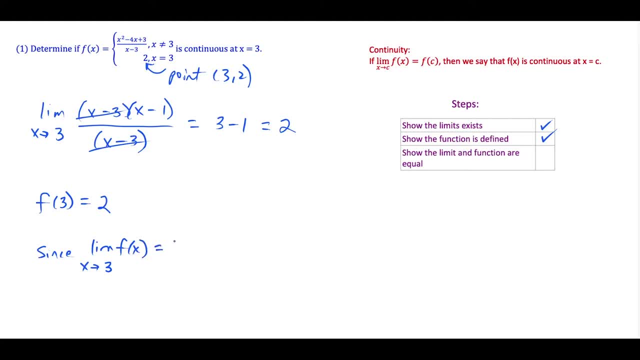 at x equals 3.. So we went ahead and showed the last step here Now, just for a little bit more insight as to like what actually happened, And if we look at a little sketch of this, this will help us understand a little bit more. Notice, all we were left with was x minus 1.. And 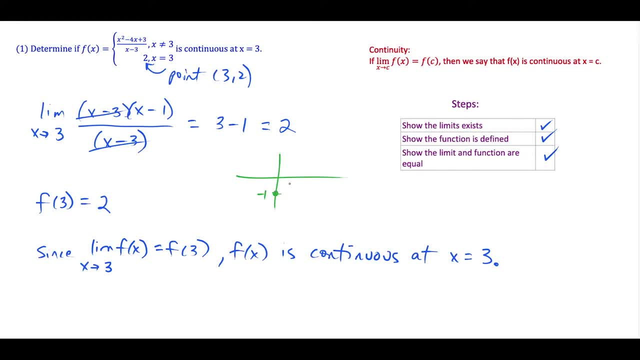 if we provide a little sketch of this, x minus 1 is a line And it looks rough. sketch something like this: So this is at the point one, and then two is out here, three is out here. So what we just found here was, at x equals two, this would go up to one, and x equals three, this is going up to. 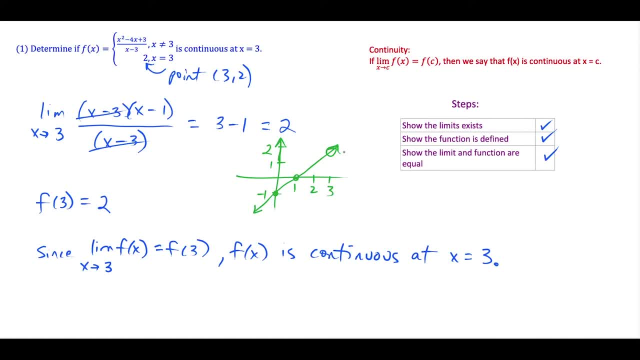 two, So temporarily, because x is not equal to three. this is a line with a hole in it here, But notice that the point three, two goes exactly where the hole in the line is, going ahead and like filling this gap, making this a continuous function If this was any other number but two. 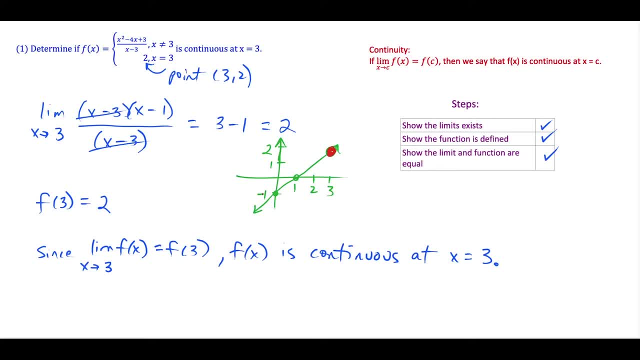 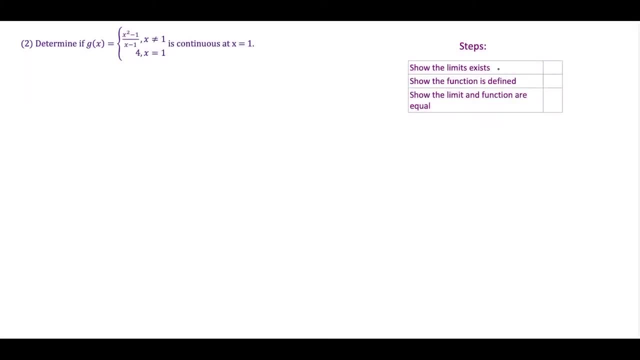 then the function would be not continuous at x equals three. But this did work out for us. So this function is in fact continuous at x equals three. So for this next example we'll start the same way. we want to show that the limit exists, But this time we want to see if g of x is. 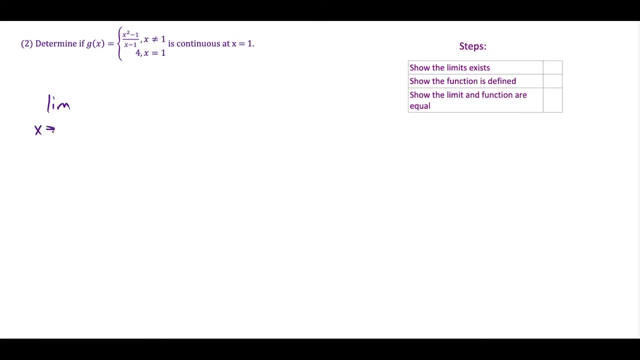 continuous at x equals one. So if we take the limit as x approaches one of g of x, we're going to factor this quadratic expression and it would factor as x plus one times x minus one and we have an x minus one on bottom. So when these cancel out, we're left with x plus one. So when we plug in x, 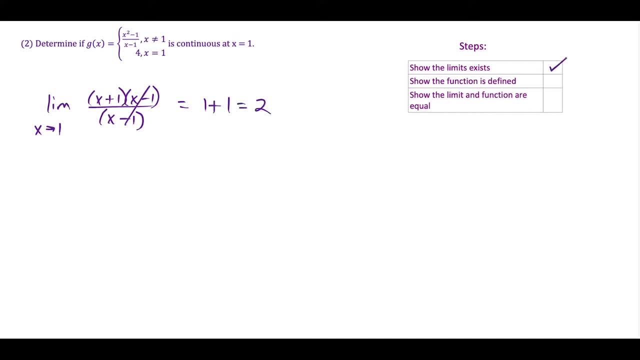 equals one. we have one plus one is equal to two. So the limit does exist. But notice this time around, if we look at the function value- and now this is for g of x, the function value at one is equal to four. So right away I would say this is not continuous. at x equals one, because the limit 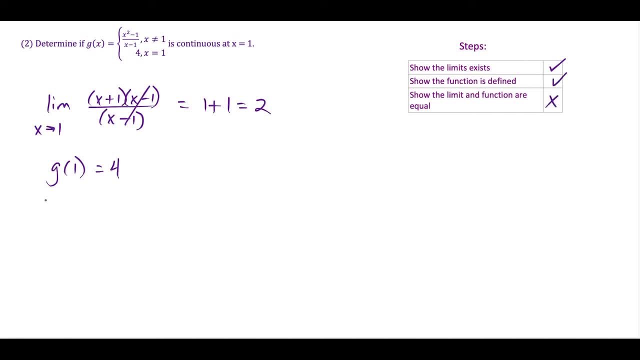 and the function are not equal. So this last step is not satisfied. If we want to investigate this a little bit more, we could just look at a rough sketch of this and see that if we look at the left over here, the line x plus one, 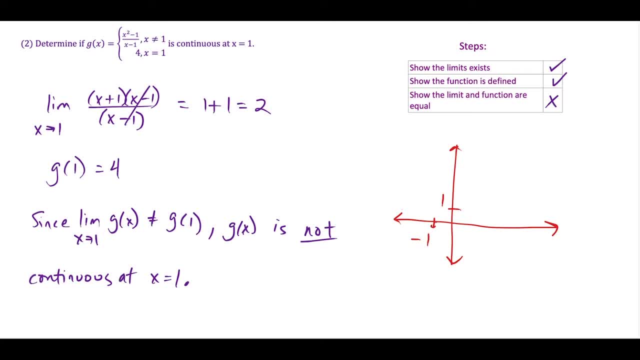 so we'll just get a little sketch here. So these would be the intercepts. So, once again, this is just a rough sketch, But notice, everything that's going on is, at x equals one, that the limit is equal to two, but the function value was equal to four. So this is a situation here where, when we once again have 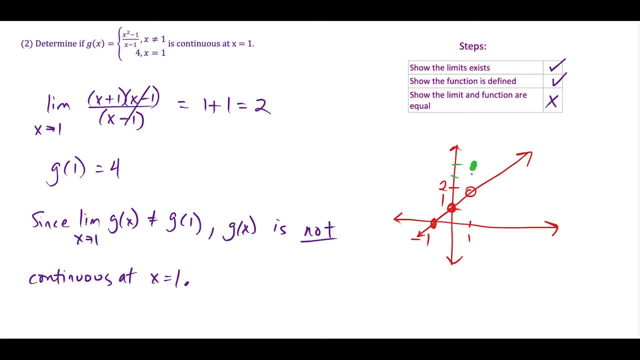 a line with a hole in it, but the function value here is up top, So this would be a removable discontinuity. If this y value here was equal to two, then this function would be continuous. But since they're not equal, we can say this function is not continuous at x equals one. So for this: 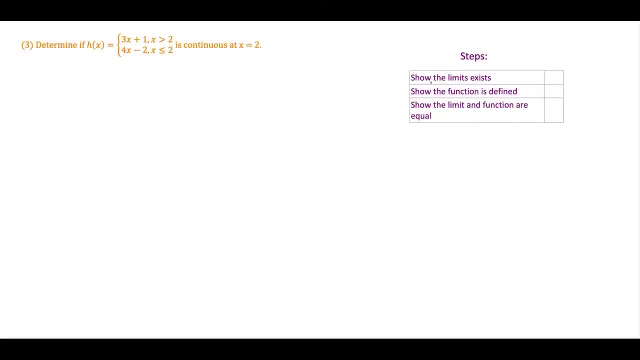 type of function. we want to show the same thing- that the limit exists, the function is defined- and show that those two things are equal. But this time around we have a slightly different piecewise function. The limit exists. it's a little bit different. Now we have to investigate what is the left side? 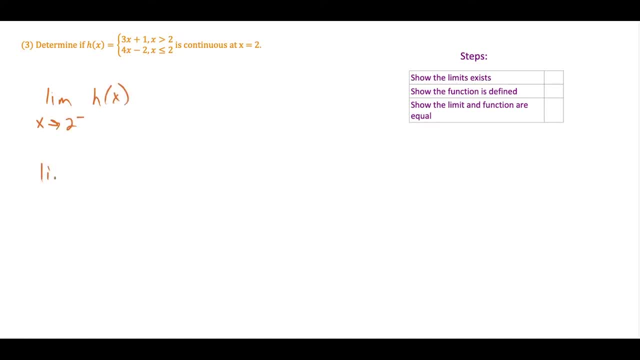 limit of h of x and what is the right side limit of h of x? So when we do this, the thought process that we should be going through is we have to associate left side with less than So. what I mean by this is, if I have some number line and the target value is, x equals two. when I think of 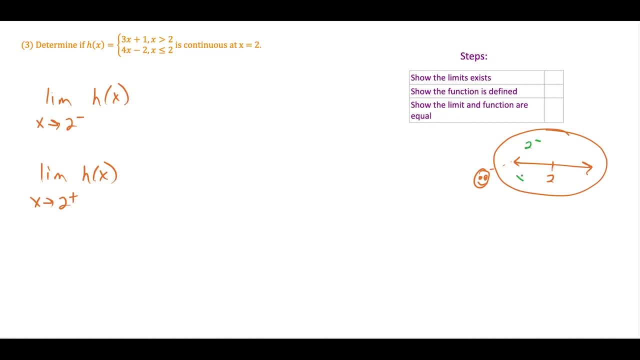 the phrase two from the left, I associate that with x less than two. So I have to associate that with x greater than two, because when I'm on the left side of two, I'm looking at values less than two, And when I'm looking at two from the right side, I associate that with x greater than two. 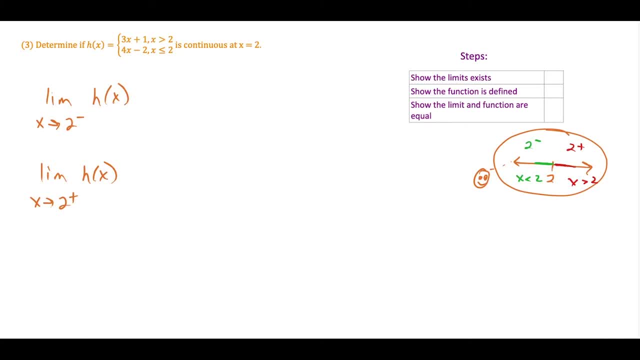 because values to the right of two are greater than two. All right, the only thing different here is- I would just throw in this- less than or equal to to match the actual question. But now, how does that help us? Well, when we want to find the limit as x approaches two from the left of h. 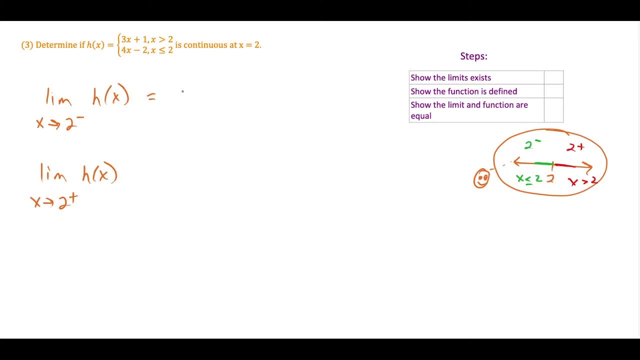 of x. we have to look at the x less than or equal to two piece And instead of doing four times two, we're going to replace that x with two And we have: four times two is eight minus two is equal to six. And then, when I investigate the limit on the right side of two, the right side of two, two plus. 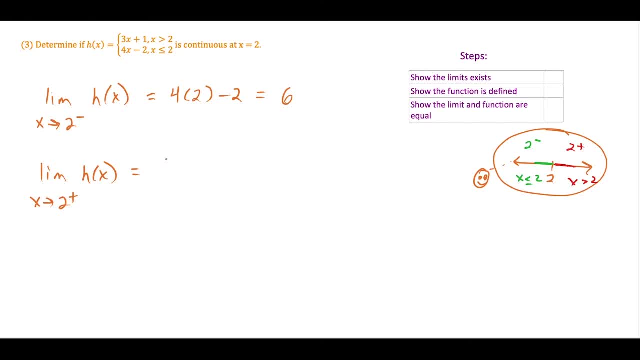 I'm looking at x greater than two, which is the top part of this piecewise function. So that's when I use the three x plus one, So I'm replacing that x value with two And this is going to give us seven. So notice right away: the left and right limits are not equal. So since the left and right 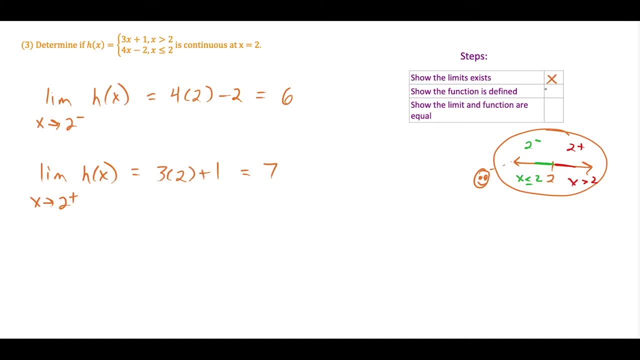 limits are not equal, this tells us the limit doesn't exist. And if the limit doesn't exist, this tells us the function is not continuous at x equals two. I should just mention something real quick. these three dots mean, therefore, it's just a. 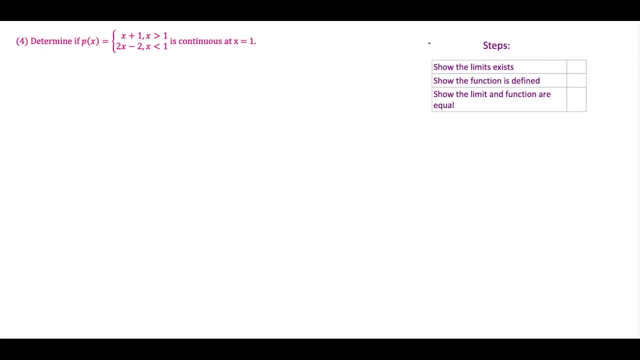 nice abbreviation when you're writing explanations in math. So for the fourth question we're going to start the same way, But this one has a little bit of a trap sprinkled into it. when I look at this right away, I automatically say that this function is not continuous at x. 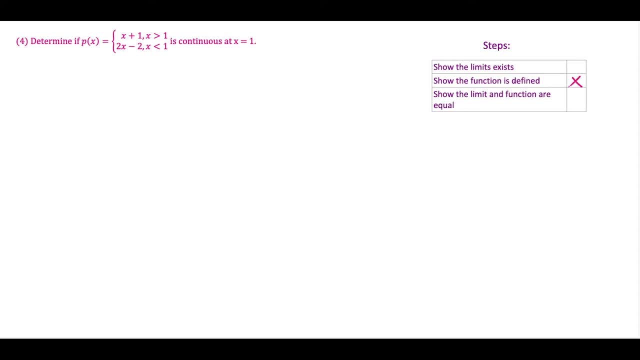 equals one, And the fast way I could say it is that this function is not defined at x equals one. Notice here that p of one is undefined because for this piecewise function we only have these intervals here, for x greater than one, x less than one, but notice none of them. 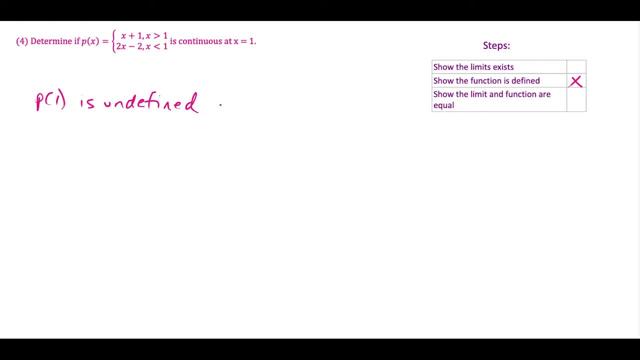 include an equal to. So, since p of one is undefined, this tells us we could say: and therefore p of x is not continuous at x equals one. Okay, so last question: here we're looking at the function q of x, the first thing we want to show. 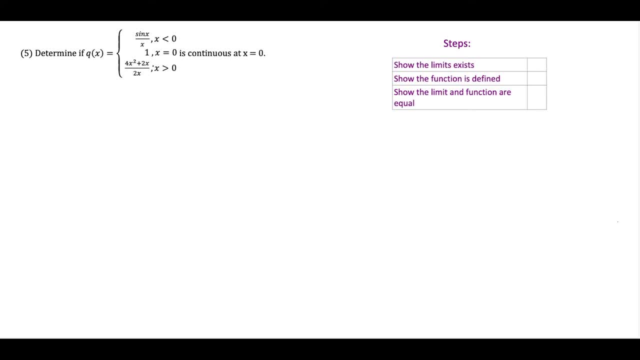 is that the limit exists. So notice this is broken into three pieces. we have x less than zero, x equals zero and x greater than zero. So if we want to show that this limit exists at zero, first thing we could look for is: what is the limit as x approaches zero? from the left. 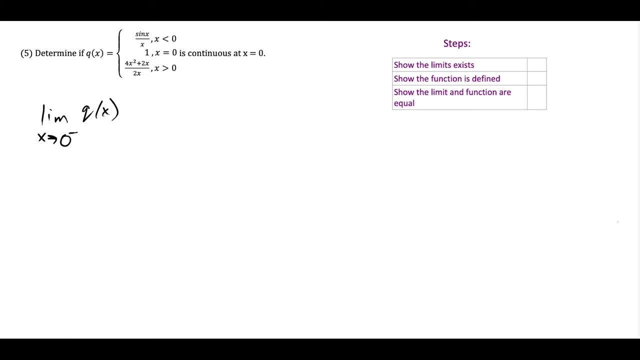 of q, of x. So if I'm looking for the left side limit, so we're looking at zero from the left, that means I'm using the x less than zero limit. So I'm looking for the left side limit, so I'm 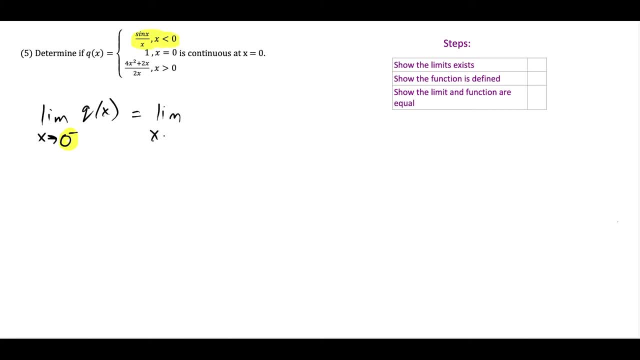 0.. So when I evaluate this, this is the limit as x approaches 0 from the left, and we're using the sine x over x piece. Now, this is a famous limit. The limit as x approaches 0 of sine x over x is equal to 1.. If you forget this, you could always use L'Hopital's rule. 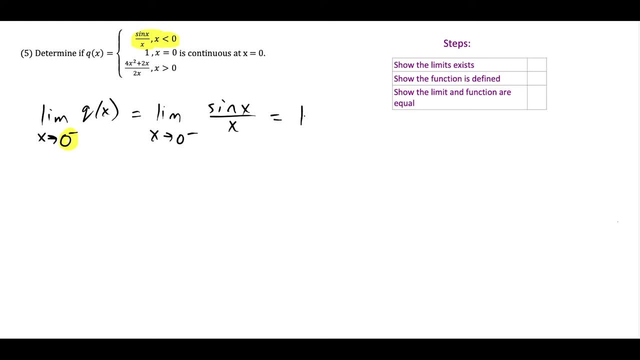 if you've learned that part of derivatives yet. But otherwise we could say this limit is equal to 1.. So now we want to find what is the limit as x approaches 0 from the right side of q, of x, And for this what we're going to do is we're going to use x greater than 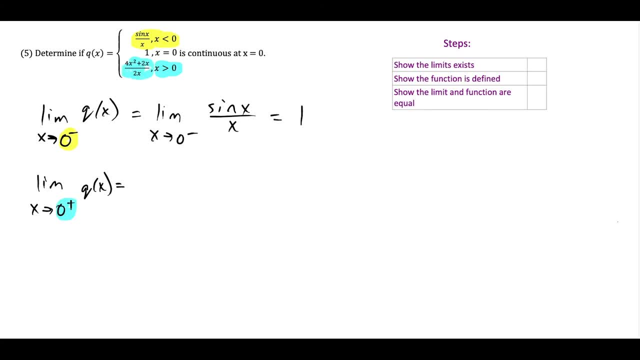 0 for 0 from the right. So we're using this piece here. So what we could do is we're going to take the limit as x approaches 0 from the right, and we're going to take this expression here and factor it On top. we have 4x squared plus 2x, So we have a greatest common factor. 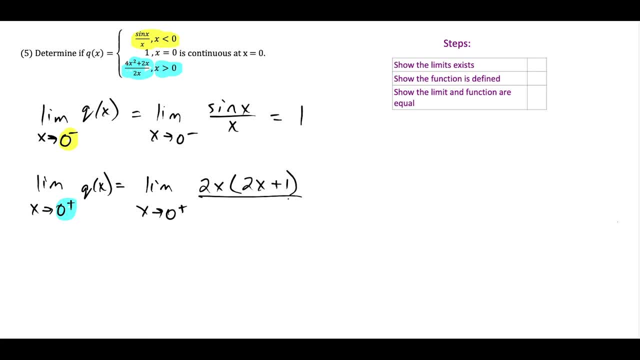 of 2x and we would be left with 2x plus 1.. And then on bottom here, we would be left with 2x. So notice: 2x over 2x cancels out. And then now, when I plug in 0, I have 2 times. 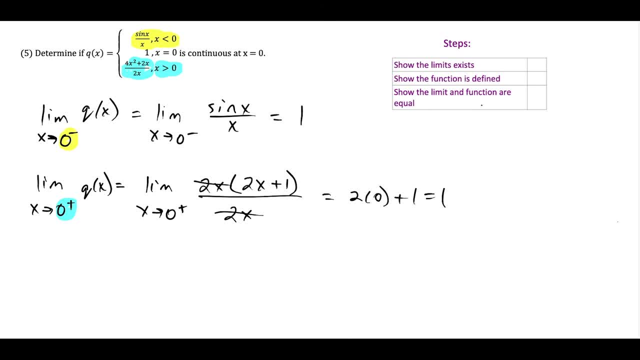 0 plus 1, which is equal to 1.. So what conclusion we can make? What we can draw from this is that, since the left and right side limits are equal, this tells us that the limit as x approaches 0 is equal to 1.. 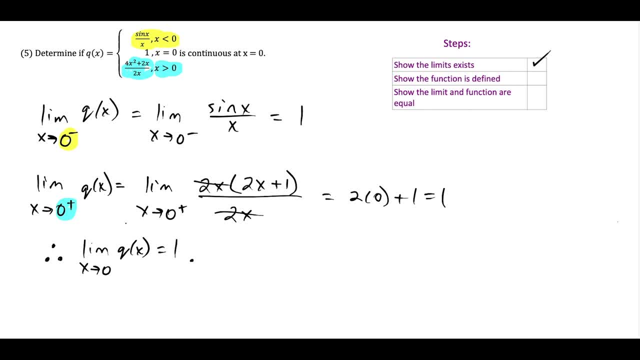 So now that we've shown that the limit exists, we can investigate the function value. So we have the limit as x approaches, 0 of q of x is equal to 1.. And now we could find q of 0 is equal to 1.. So what this tells us? we have, the limit exists, the function is defined. 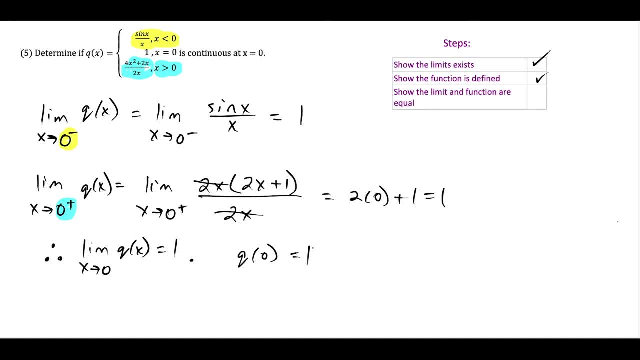 and the limit, which is equal to 1, is equal to the function value, which is equal to 1.. So this tells us that q of x is in fact continuous at x equals 0.. Okay, well, this is going to conclude this video on determining continuity of piecewise functions. 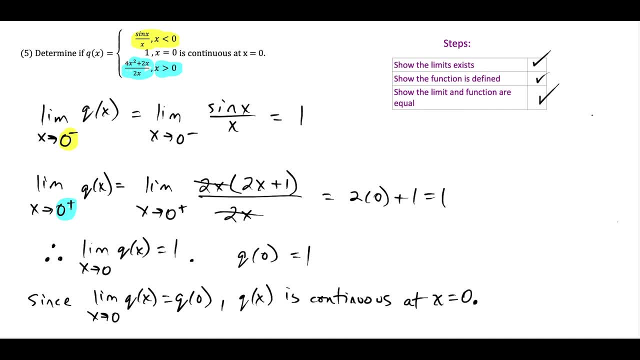 If you found this video to be helpful, please like and subscribe. It really helps me grow the channel And if you've got any requests, just leave the topics you want me to cover in the comments section below. And thanks for watching.